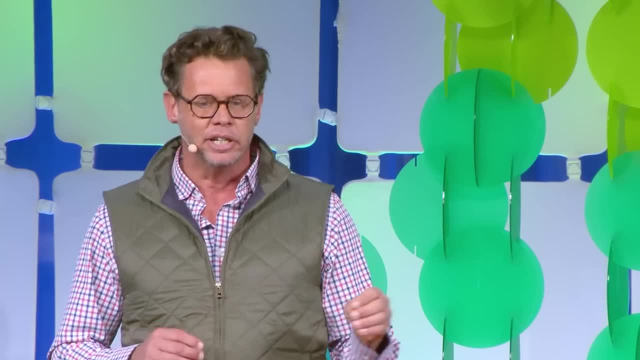 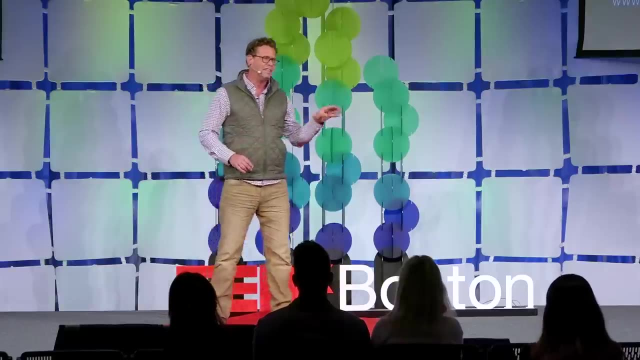 embracing natural systems to guide our design and innovation, but specifically how biomimicry can be leveraged to use ecological processes to design systems and facilitate systems change. But usually, before you arrive at biomimicry, you ask yourself one simple question. 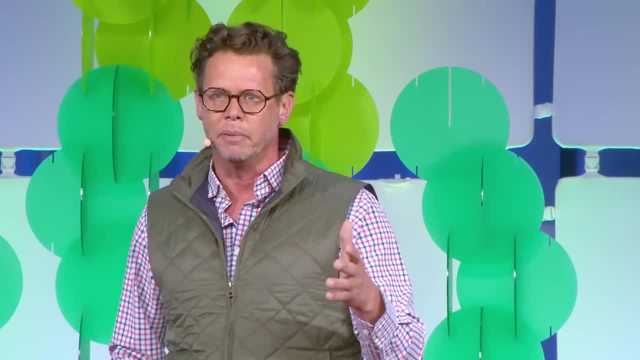 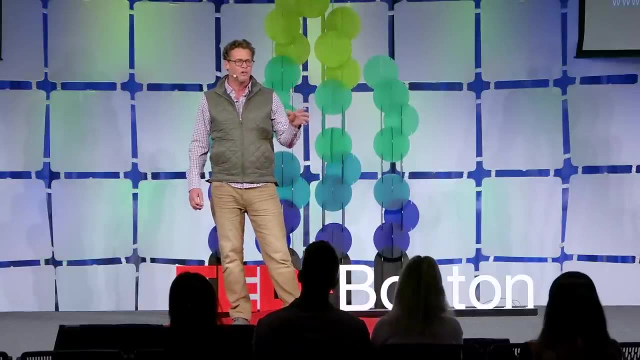 Does the earth have a solution to the thing you perceive to be a problem? Now, let's be clear: The earth may not perceive it as a problem, But there may be a solution within nature's technology that solves your problem. If yes, then before rushing to innovation or concrete or ego, look to biomimicry. How would 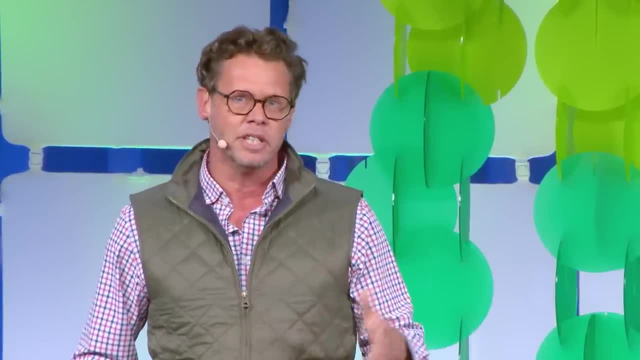 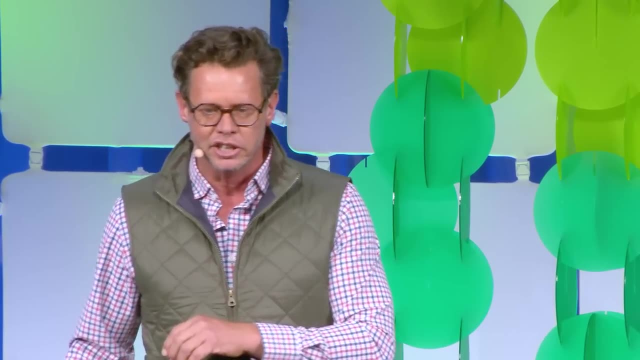 nature solve this? And can we or are we supporting those systems to the best of our ability? Some we're not. And yes, I did say nature's technology, Natural systems are inherently technology. And again, I have good news. I know you didn't expect good news to be the 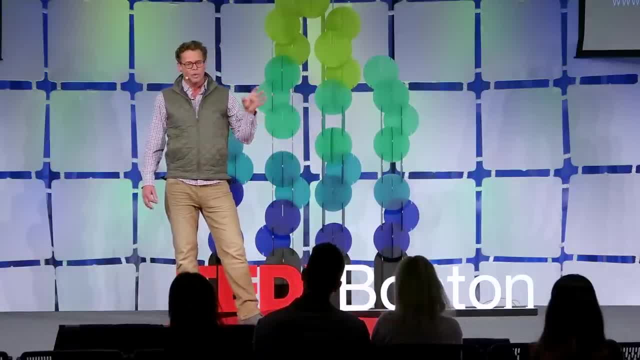 theme of this talk today. but spoiler alert, it gets better. When many people think of technology and the hollowed ground of our institutions or in the innovation hub of Silicon Valley, they often think of human-driven tech development. In these cases, the time to develop the technology. 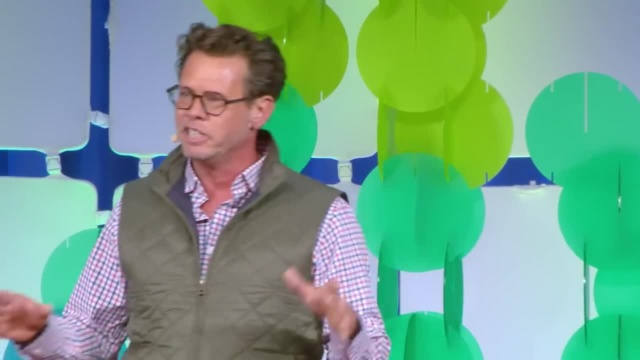 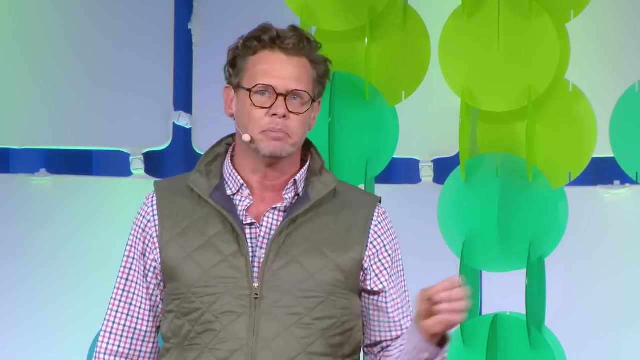 and the QA that follows are often the most expensive elements, not to mention coming up with the IP and the ideas in the first place. Well, when looking to nature's technology and biomimicry, the QA has been completed over millennia, fine-tuned thousands of years. 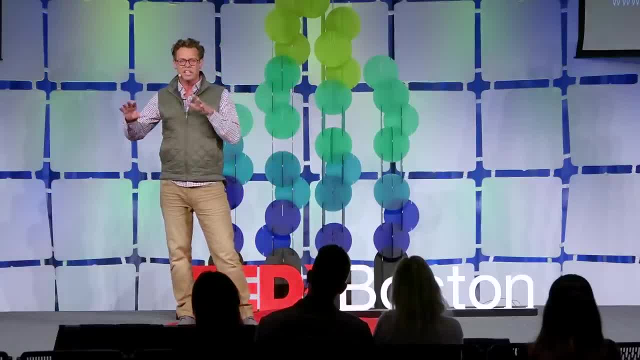 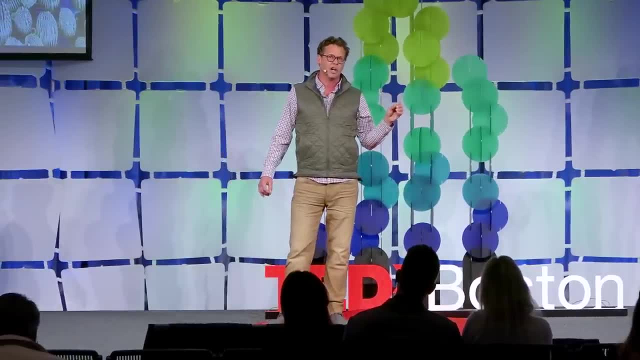 of engineering effort. The data sets the proof. it's already there, ready to be processed. It always has been So. back to soil. What do we know? Soil is the second largest carbon sink on the planet, behind the ocean, ready to reclaim its role in biosequestration at 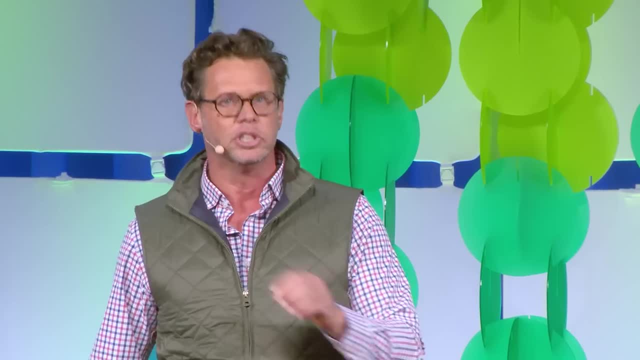 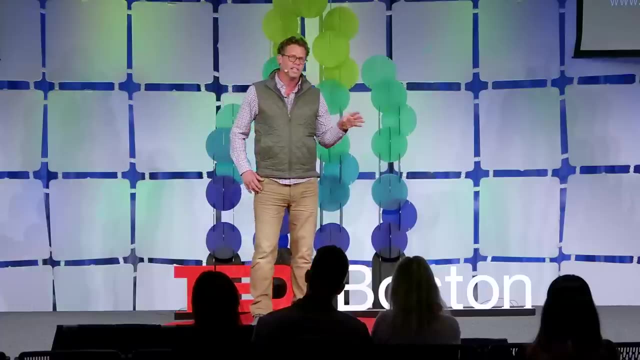 scale, And it bears note that healthy soil practices also support ocean health. Now the soil-to-ocean relationship deserves a talk dedicated on its own, so more on that another time, When focusing on agriculture. if we convert monoculture tilled land to low-till, 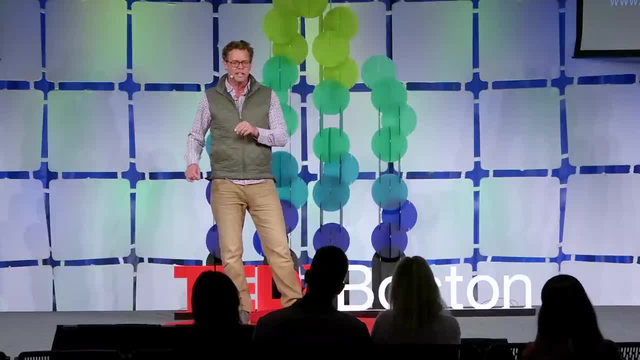 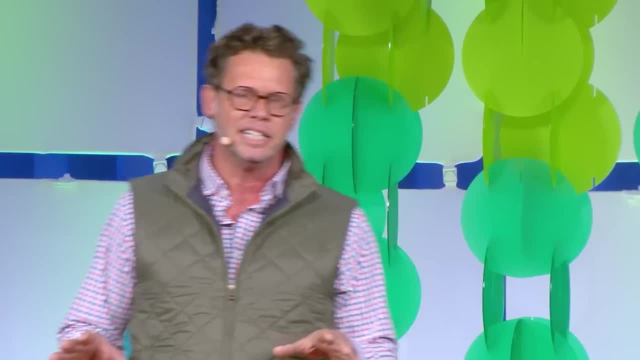 no-till regenerative practices. that land alone can take as much carbon out of the air annually as we emit annually. as I said previously, However, let's not lean on that detail to get to net zero. Why? Because soil is in a unique position to be the greatest partner. 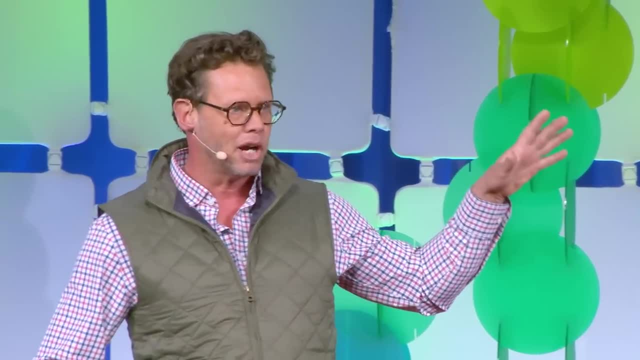 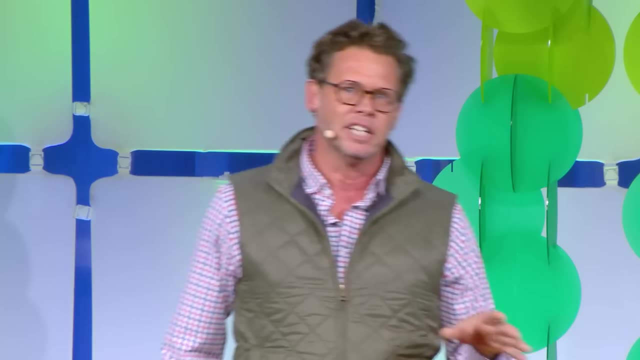 that we have to achieve drawdown. You know that legacy load of carbon that we've had in the atmosphere thus far. It's still up there. It needs to come down. We need a partner in that. But what else is happening alongside this? carbon sequestration, or rather biosequestration? 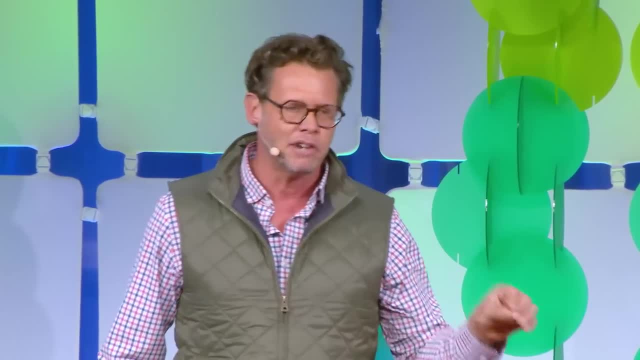 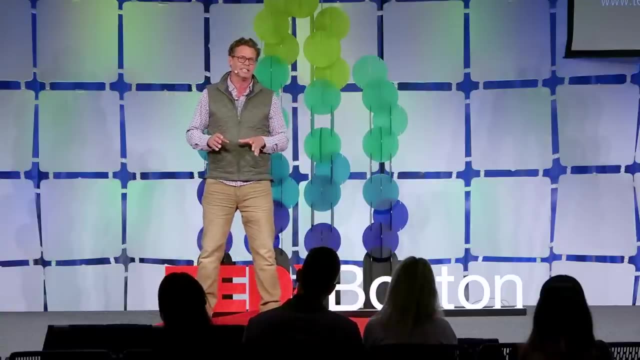 through. we be more specific. Well, healthy, carbon-rich soil means healthy microbes, which we now know directly relate to enhanced nutrition. Here's a fun fact: There's now a handheld spectrometer being tested, usually a big, expensive machine that only exists in a lab or university. 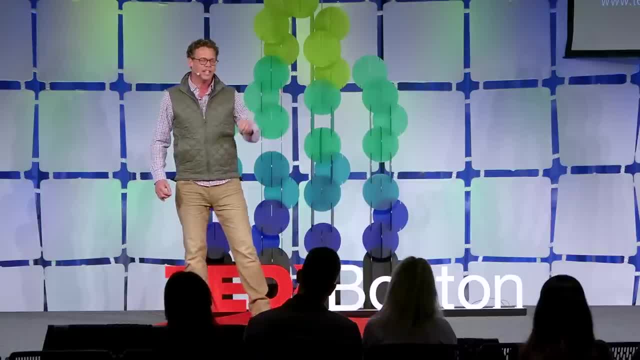 This spectrometer can fit in your pocket and measure nutrient density. You can take it to a supermarket. hold up to one carrot versus the next. Both may be organic and one may have 90 times more nutrients than the other. This directly ties back to the microbial environment. 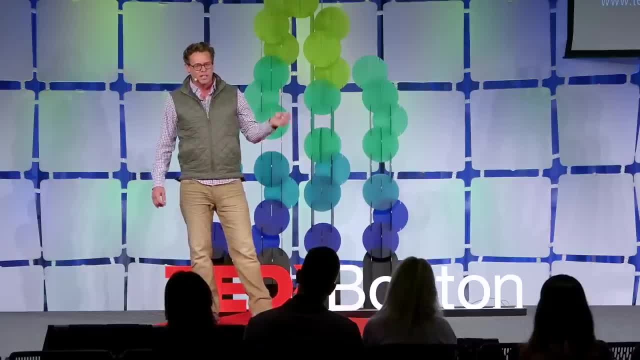 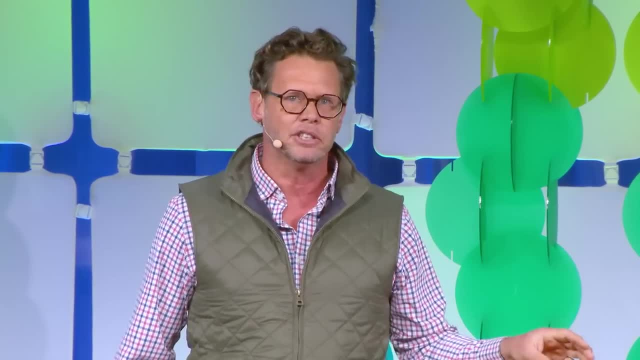 in which it grew the soil. So, along the way to carbon sequestration, to scale, you get food security and resilience and equity and so much more. These regenerative practices also expand the soil so it can hold more water, fending off both droughts and floods. Yes, there's more When you're not. 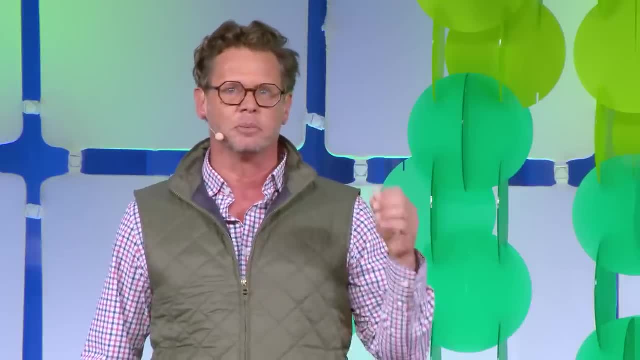 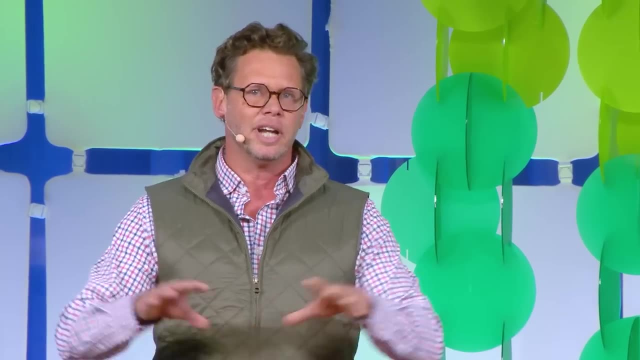 telling the land. you're protecting it with cover crops. This cools the ground. It supports transpiration and additional ecosystems and pollinators and more. If we make these things a priority, this all can happen relatively quickly, But of course it will take effort. 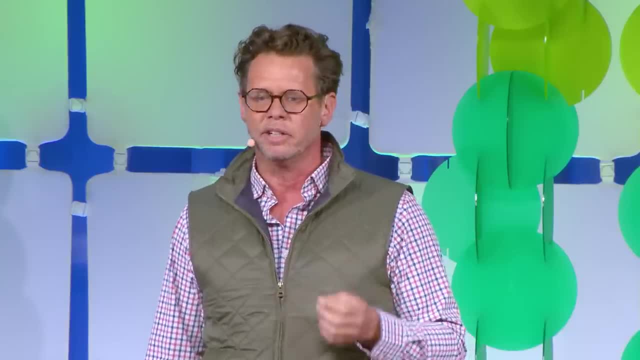 But in the context of what is at risk, that effort counts. If we make these things a priority, this all can happen relatively quickly, But of course it will take effort. But in the is at risk, that effort is minimal. Now it bears note, these practices that I'm talking. 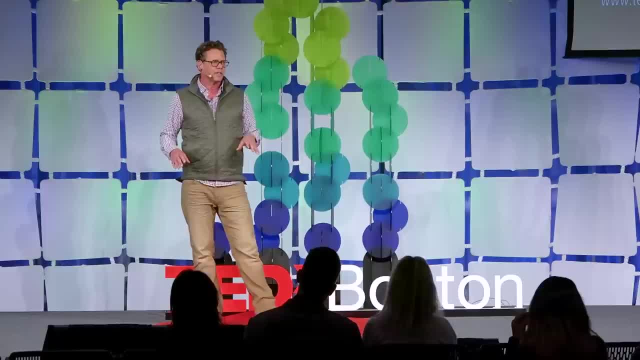 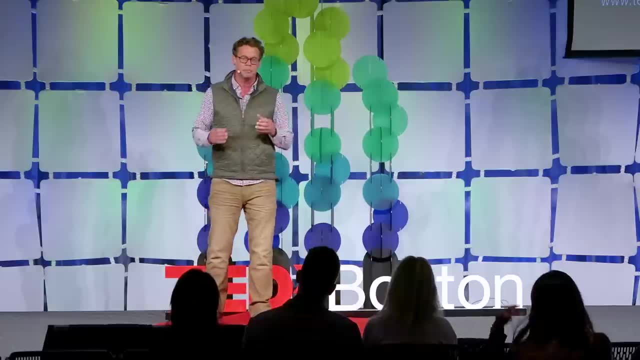 about here today are not new for humanity. Indigenous people globally have been practicing them for thousands of years. For generations, these communities have been asking for other people to pay attention, to listen to the lessons the earth has for us. Alas, this is. 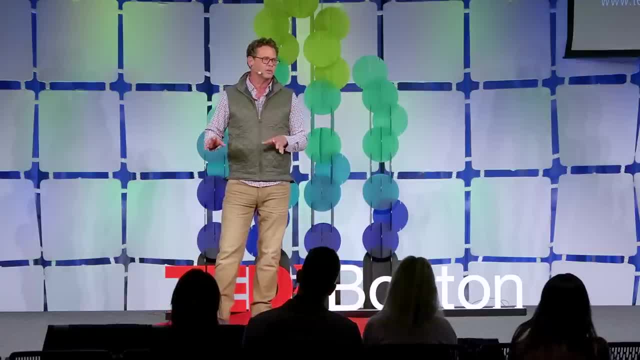 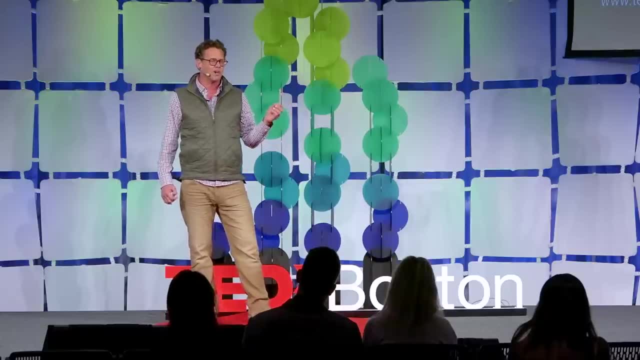 a whole other conversation that needs to be had more broadly, on its own, in the context of reconciliation and systems change. And yet this brings me to the most powerful part of soil as a primary climate solution, its intersectionality As discussed. soil-related. 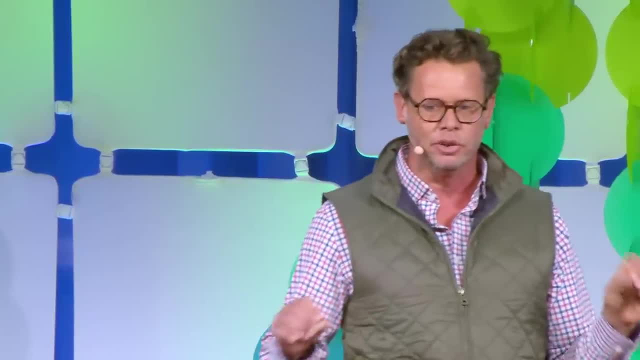 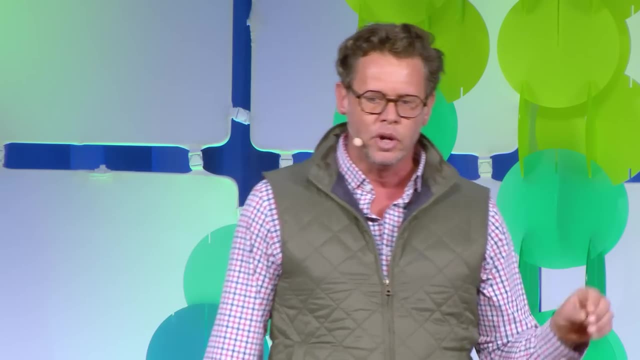 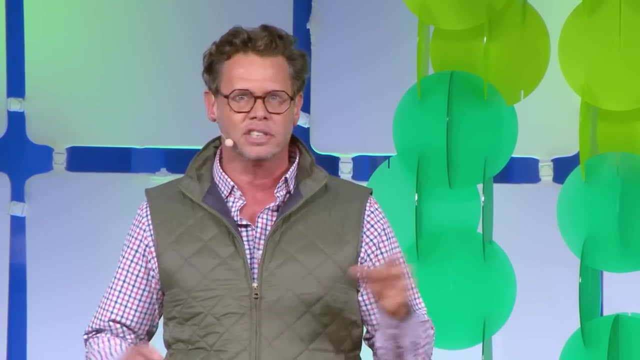 opportunities touch upon so many communities and interests. it may be in our greatest unifier available. We can embrace multidisciplinary approach needed to achieve climate change at scale With soil. independently or together, we can work toward the intersectionality of social, racial, environmental justice. We can clearly see the confluence of art science. 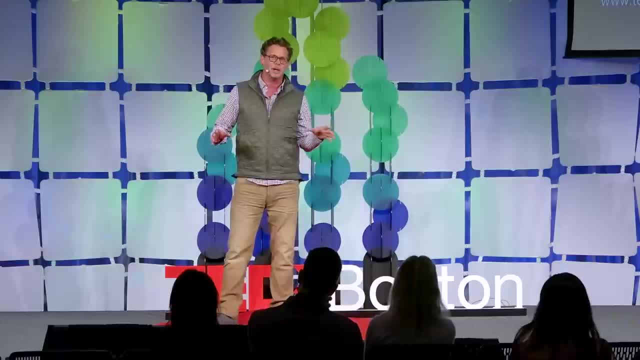 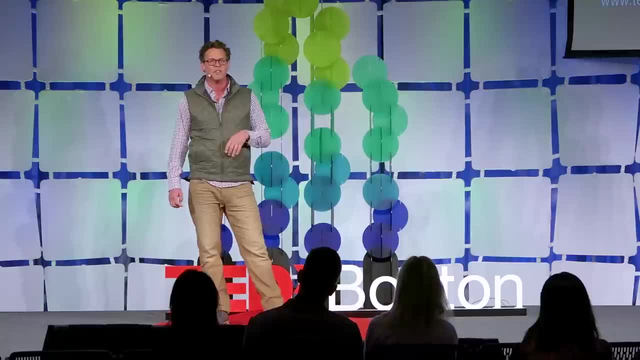 technology and policy. We can remove the myth of externalities by embracing traditional capital and natural capital holistically, especially when considering that nature-based markets are seven trillion dollars a year. With soil and other solutions, we can achieve drawdown. For this there is. 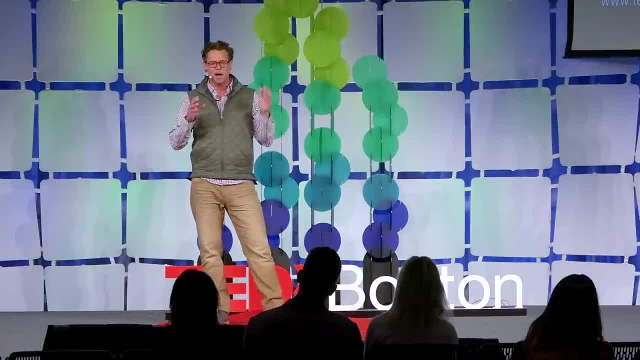 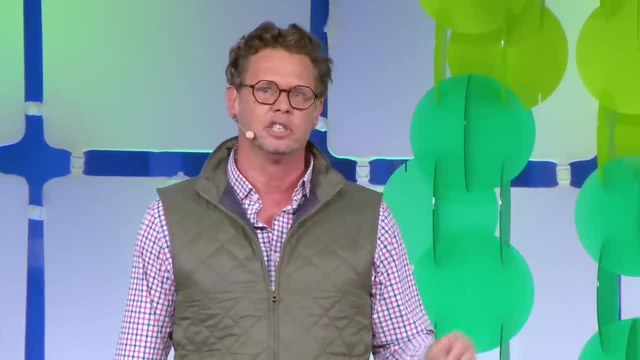 actual plan, Given the scale of the challenge and the democratized and distributed nature of the solution. we need to activate, educate and engage at scale. We need regional centers to support municipalities and populations as uniquely needed for their bioregion and 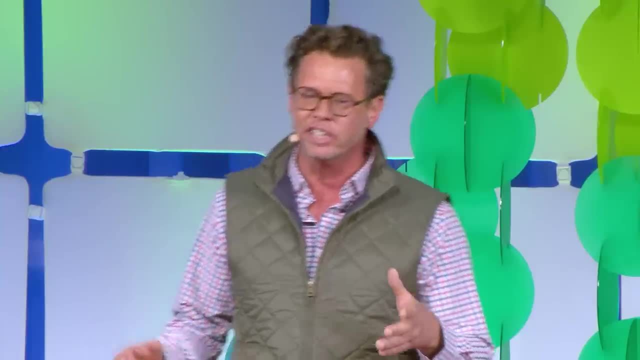 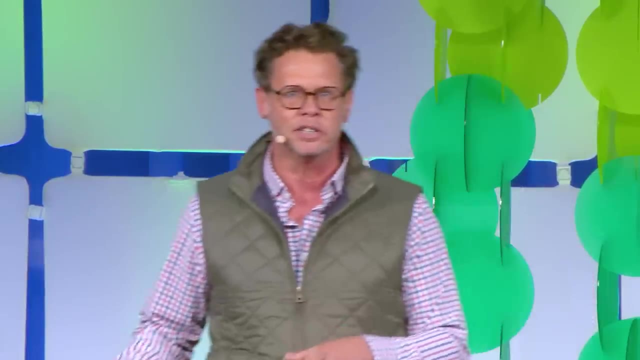 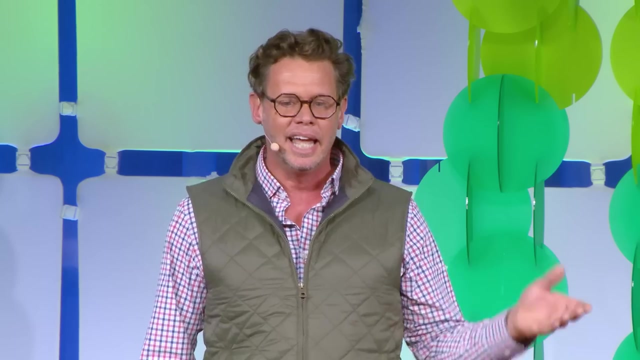 watershed, to train people, to support communities, to provide resilience. We are in a climate crisis And, pragmatically, all crises require first responders distributed with information, resources and technology, led by local populations in alignment with their ecosystems. And again, 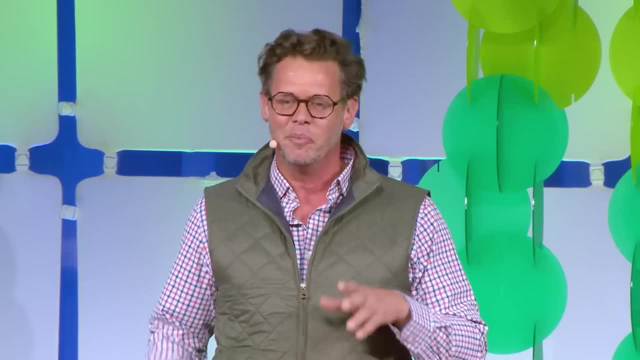 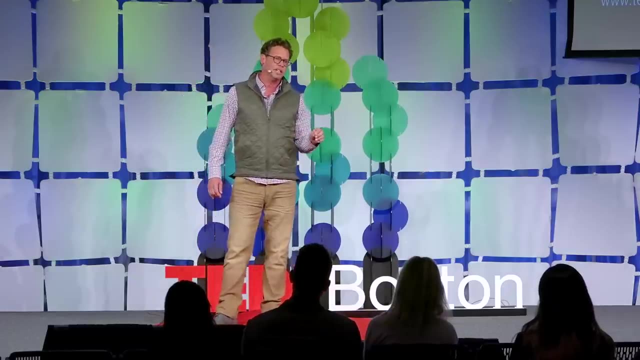 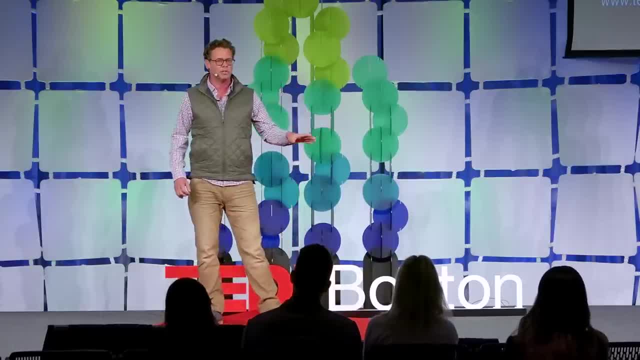 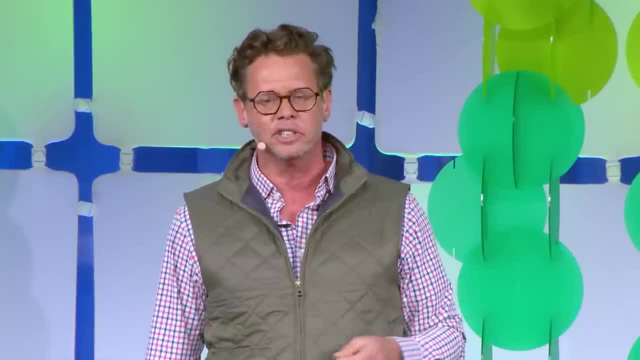 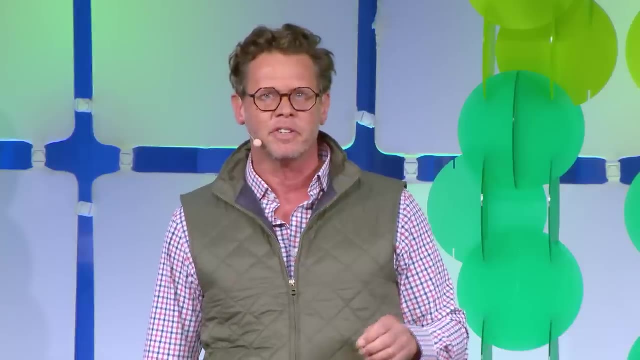 From increasing the health and prosperity of rural communities to waste stream capture and closed-loop systems, from workforce development to early childhood brain development. So what to do? You can support legislation that centers on natural systems. You can help transition harmful practices. You can steer your municipality to both soil and improve water systems. You 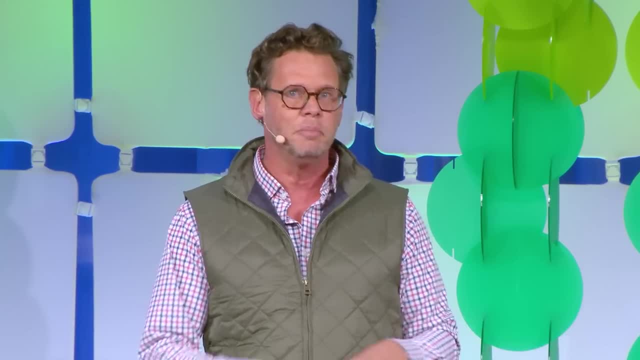 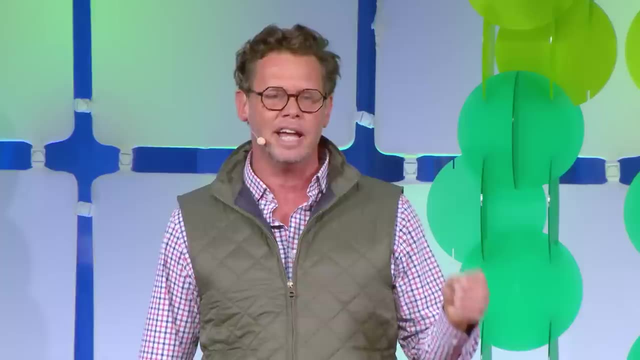 can start an urban farm, a food forest or a soil science center. You can build AI that enhances soil biodiversity, and so much more. Or maybe you can do sustainable finance, seeking globally scalable net-new ESG projects with measurable carbon, biodiversity and nutrition impacts. 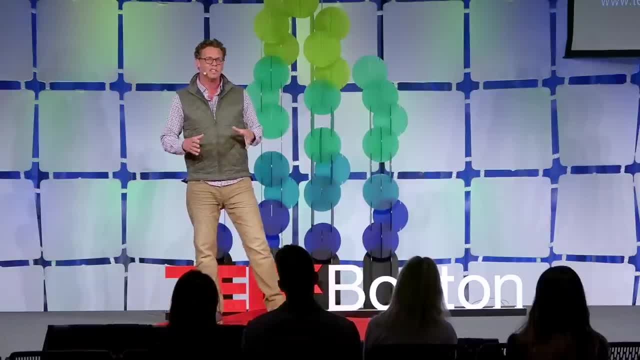 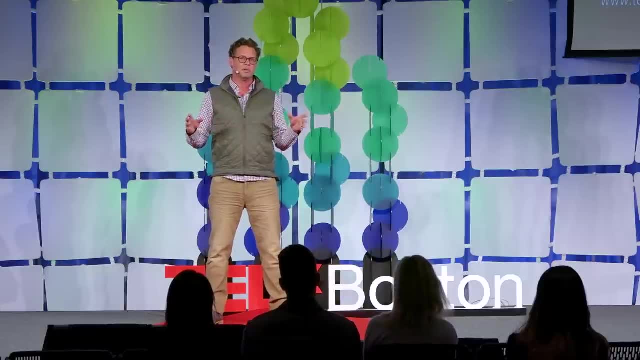 Remember how I said, soil can change my life. Well, when I learned these things, I pivoted my entire life to help co-found the REAP Climate Center, And we've already touched the lives of thousands of people. We're working towards all of these things that I spoke about here today. 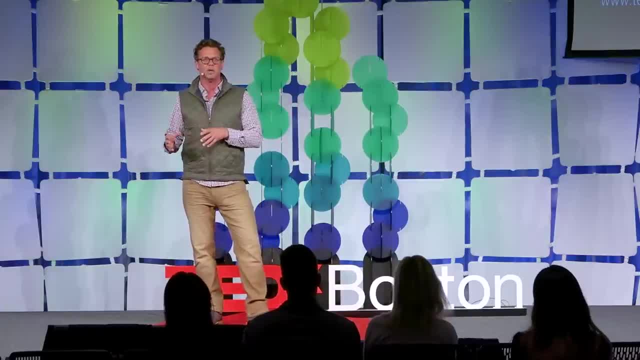 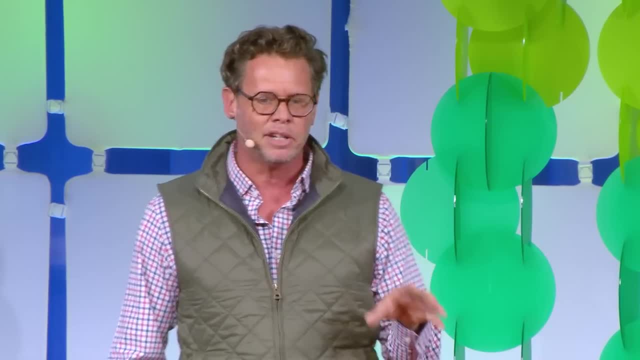 And, whenever possible, we lead with curiosity and playfulness. We're focused on soil science, regenerative systems, with an overarching goal to onboard people into climate engagements. Our half-mile-long campus on an island in the middle of the San Francisco Bay hopes to be a template for many more centers to come globally.